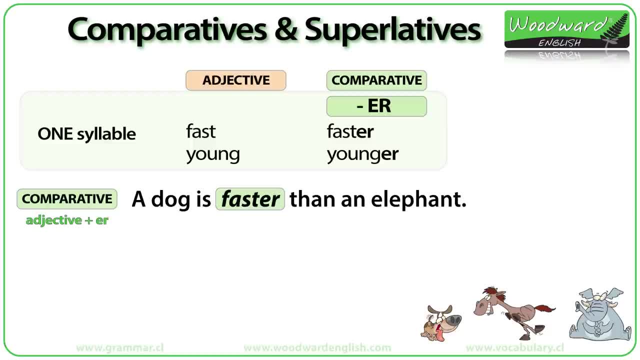 YOUNGER. Look at the example again. A dog is faster than an elephant. We say FASTER and not MORE FAST, as you do in some other languages. Also, it is important to use THAN after the comparative Faster than, slower than. 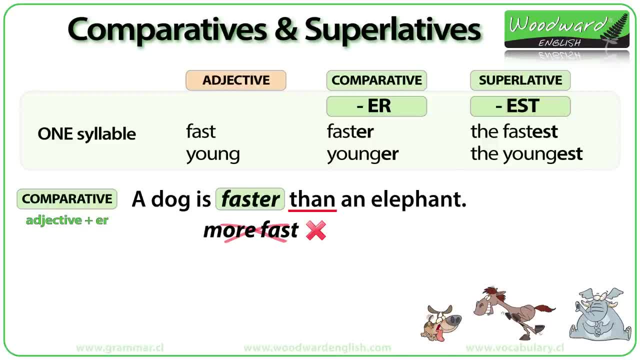 Younger than To make a superlative. we add EST to the end of the adjective. Fast becomes the FASTEST, Young becomes the YOUNGEST. It is important to have the article THE before the superlative. The horse is the FASTEST. 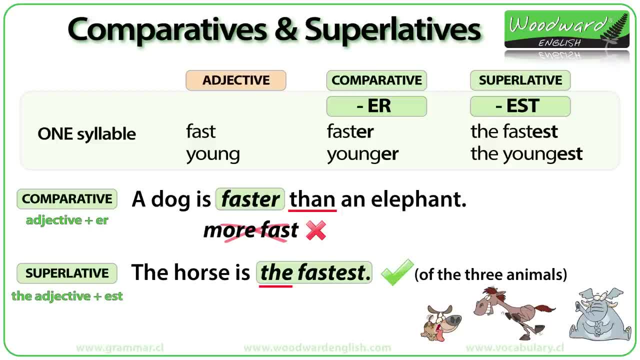 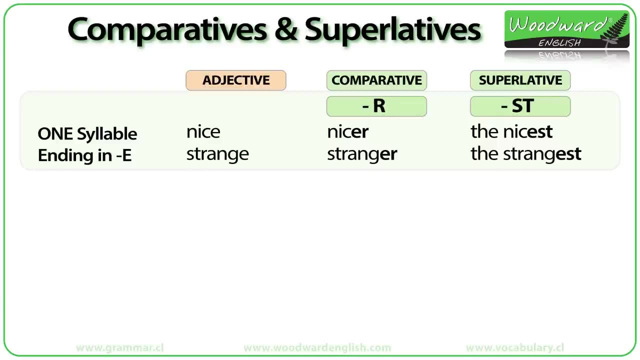 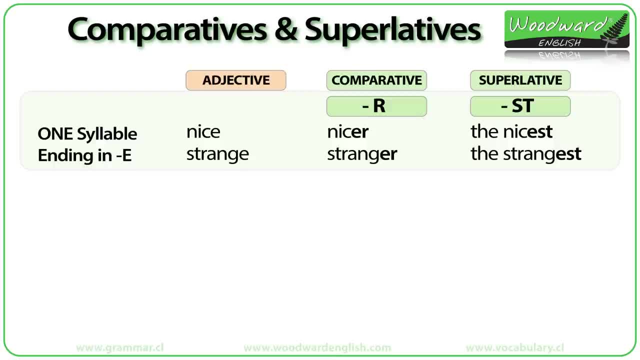 we just add an R to the end of the adjective to make it a comparative. The adjective NICE becomes NICER, The adjective STRANGE becomes STRANGER, And for a superlative just add ST, So NICE becomes THE NICEST. 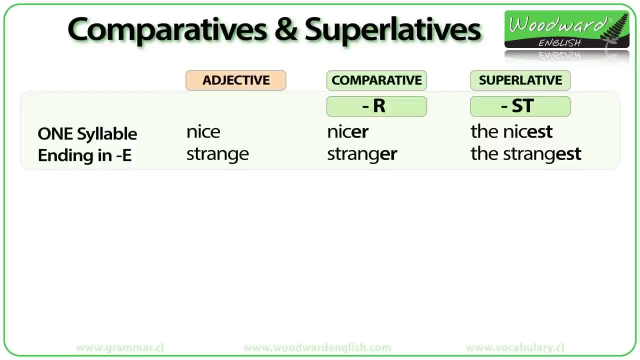 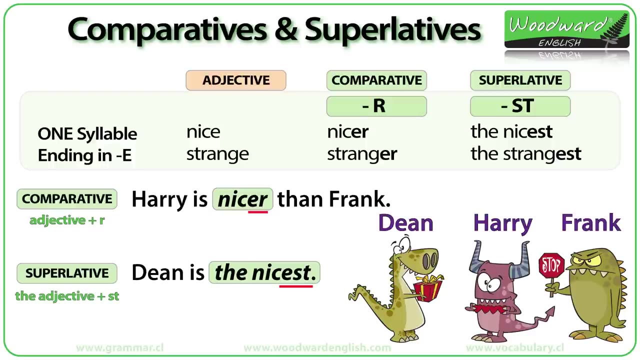 STRANGE becomes THE STRANGEST. Look at these three monsters: Dean, Harry and Frank. Harry is NICER than Frank. Yes, Frank looks like a grumpy monster, But of the three monsters, I think Dean is the NICEST because he has a gift for you. 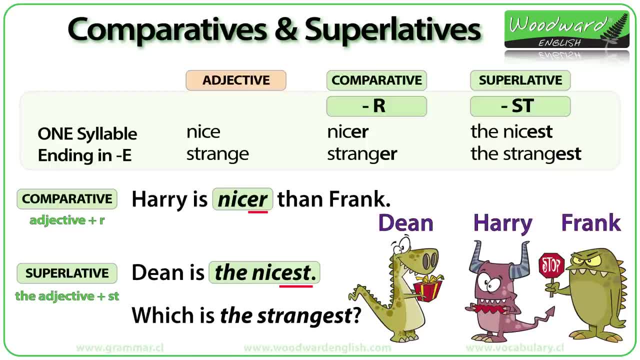 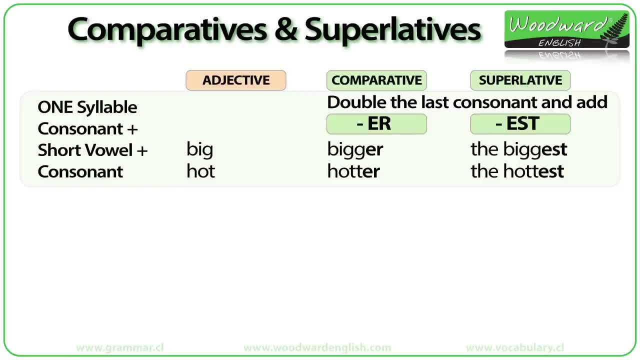 Of the three monsters? which is the STRANGEST? Yes, Frank is the NICEST. When an adjective has one syllable and ends in a consonant plus a short vowel plus a consonant such as BIG and HOT, we double the last consonant and add ER for the comparative and EST for the superlative. 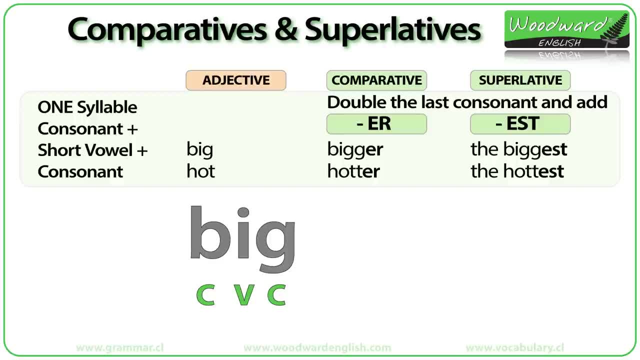 For example, BIG ends in a consonant B, a short vowel I and another consonant G, So we double or make two of the last consonant With the word BIG. the last consonant is G, So we need two Gs. 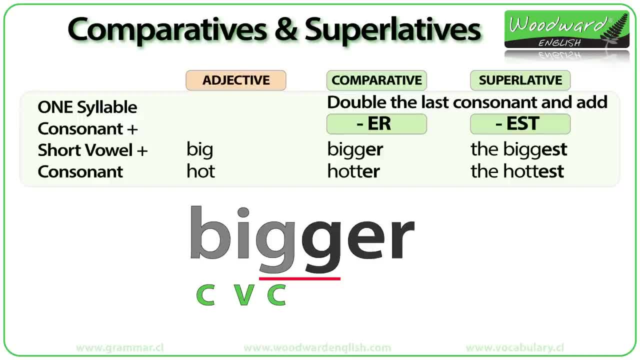 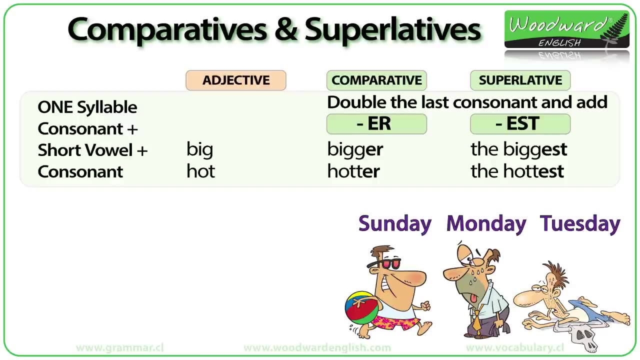 BIG becomes BIG, BIG becomes BIGGER with two Gs. The superlative is BIGGEST also with two Gs. Look at the weather on these three days: Sunday, Monday and Tuesday. How can we compare these three days using the adjective HOT? 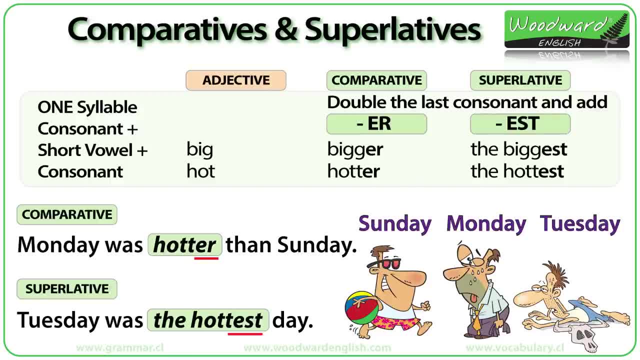 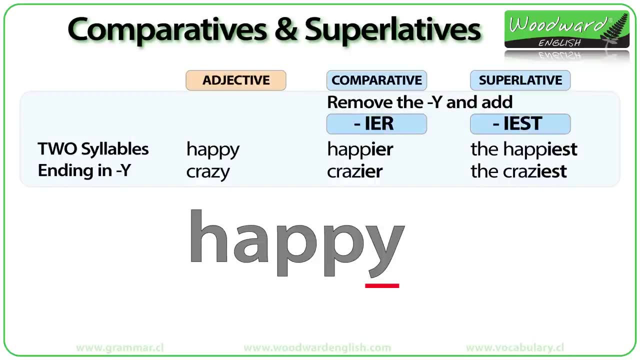 Sunday was HOT. Monday was hotter than Sunday, But Tuesday was the hottest day. When an adjective has two syllables, such as HAPPY or CRAZY, and the adjective also ends in the last consonant, so ends in the letter Y. 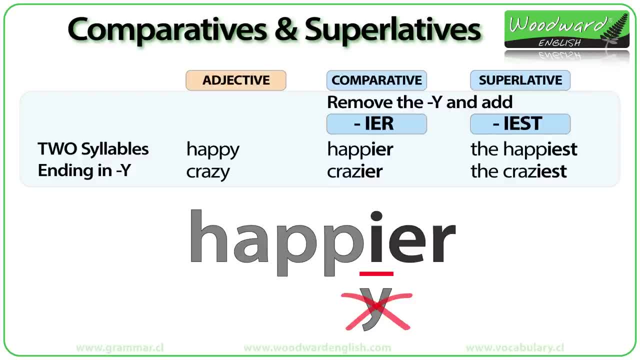 we remove the Y and add IER for the comparative, So HAPPY becomes HAPPIER For the superlative. we also remove the Y and we add IEST, So HAPPY becomes THE HAPPIEST, CRAZY becomes CRAZIER and the CRAZIEST. 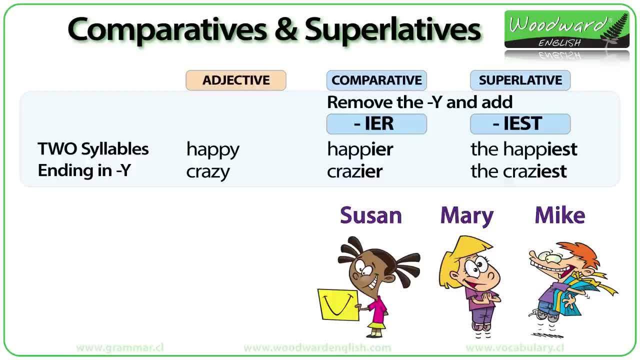 Here are three children: Susan, Mary and Mike. How can we compare these three children using the adjective HAPPY? Mary is HAPPIER than Susan. Mike is the HAPPIEST When an adjective has two or more syllables. 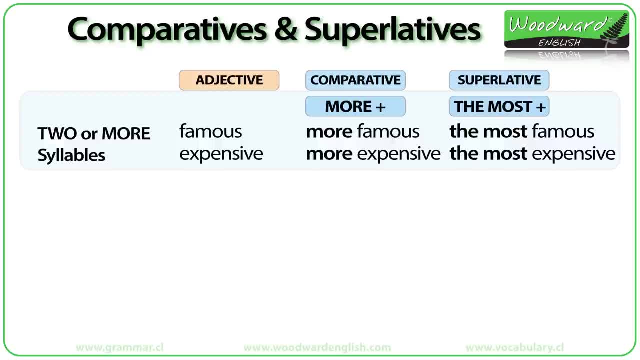 we do not add ER or EST to the end of it. The adjective FAMOUS has two syllables: FAMOUS, So we cannot say FAMOUSER, No, it doesn't exist For comparatives. we use the word MORE before an adjective with two or more syllables. 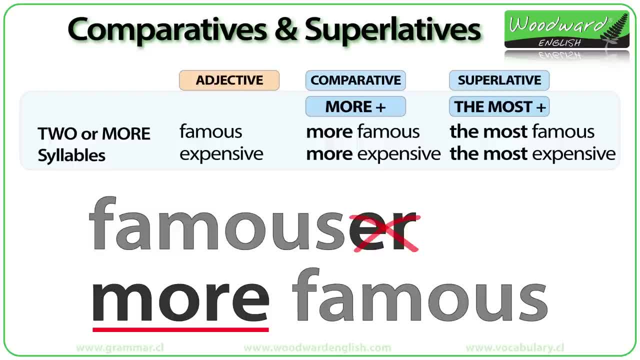 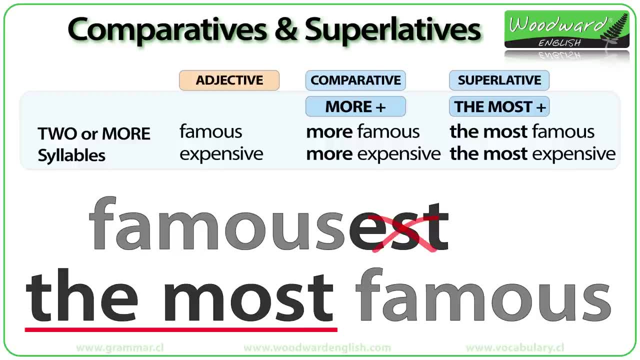 So FAMOUS becomes MORE FAMOUS. For superlatives we use the words THE MOST before the adjective, So FAMOUS becomes THE MOST FAMOUS. EXPENSIVE has three syllables: EXPENSIVE, So EXPENSIVE becomes MORE EXPENSIVE. 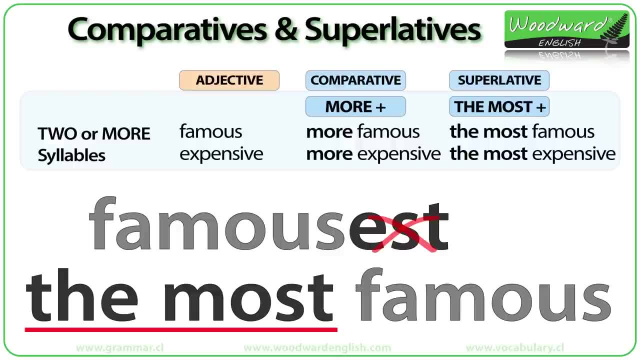 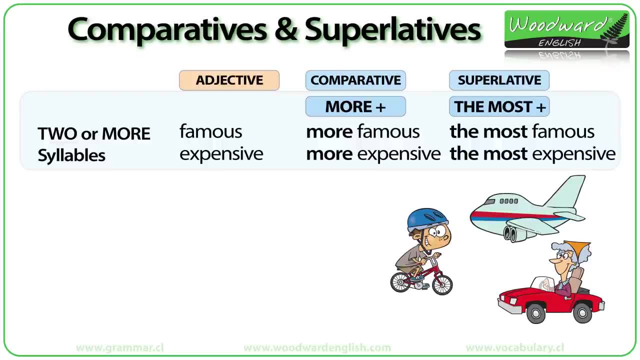 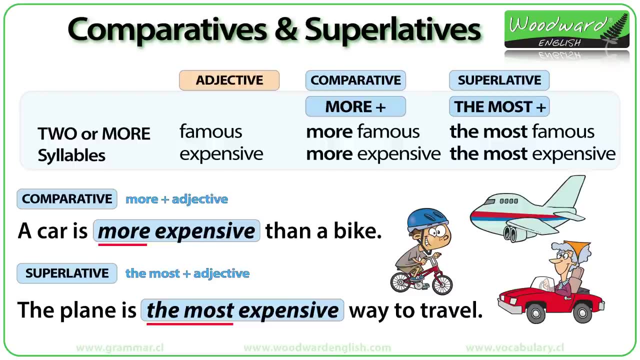 and THE MOST EXPENSIVE. Let's compare a bike, a car and a plane as ways of traveling. How can we compare them? using the word EXPENSIVE? A car is more expensive than a bike. The plane is the most expensive way to travel of the three. 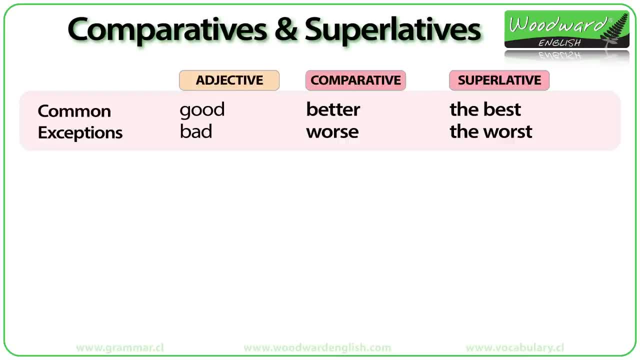 Of course there are always exceptions. in English, Two common exceptions are the adjectives GOOD and BAD. With GOOD the comparative form is BETTER and for the superlative form we say THE BEST. For example, You are a better singer than John. 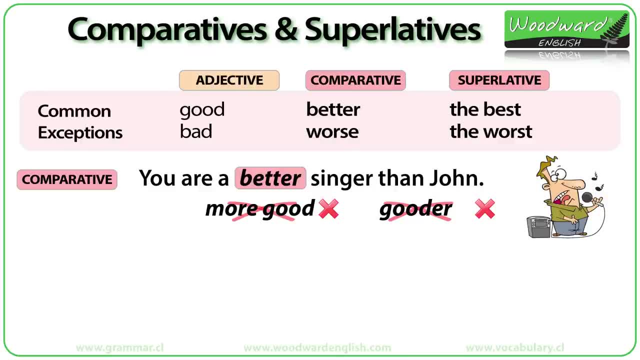 Yes, We do not say MORE GOOD No. And we do not say GOODER No. We say BETTER With BAD. the comparative is WORSE and the superlative is THE WORST. For example, It was the worst decision she had ever made. 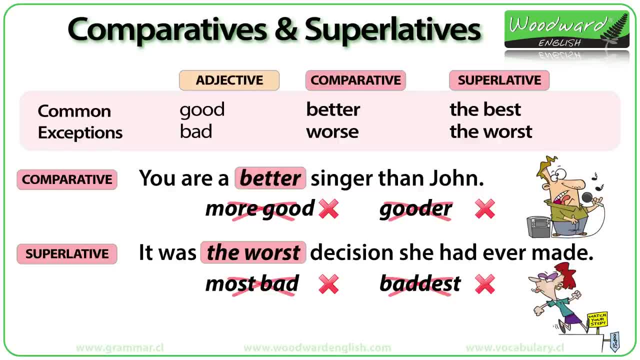 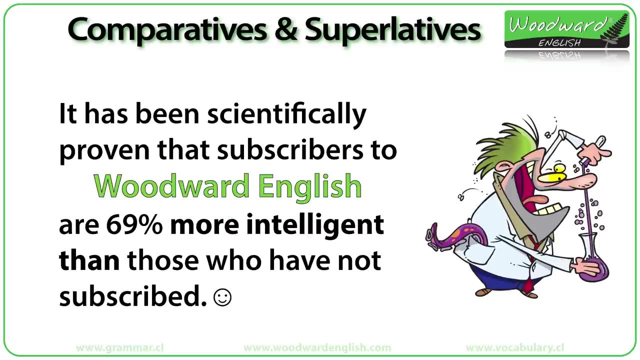 We do not say MOST BAD or BADDEST, No, We say THE WORST. There are more exceptions, such as FAR and LITTLE, but we will see these in another video. Thanks for watching this video and remember to subscribe to our channel.